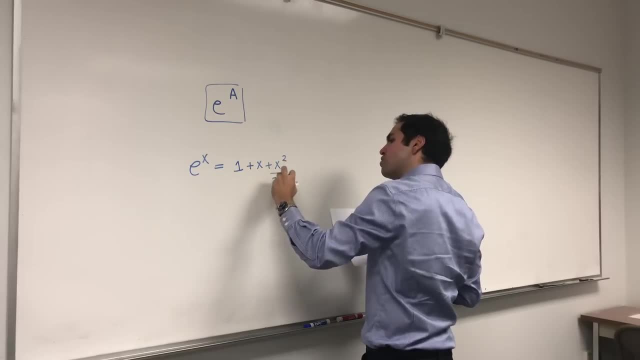 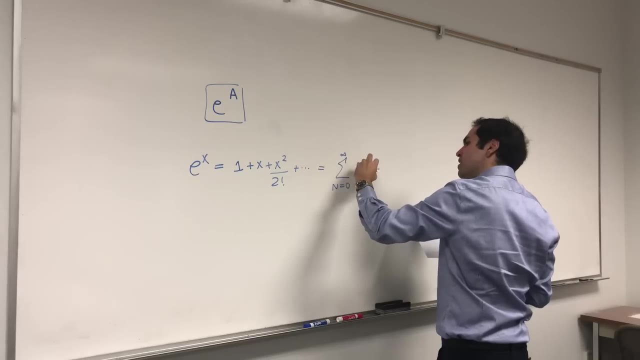 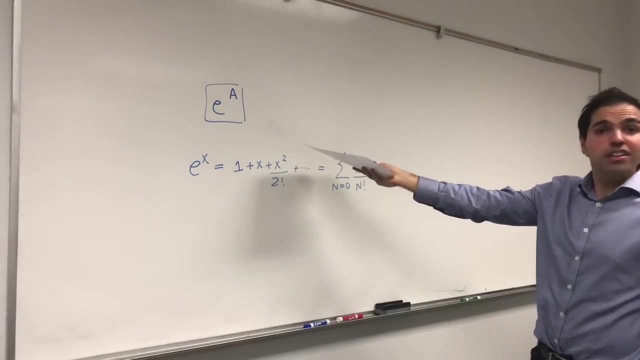 is 1 plus x, plus x squared over 2, factorial plus dot dot dot, which is the sum from n, from 0 to infinity, of x to the n over n factorial. Well, we can do the same thing for the exponential of a matrix. It's defined by almost the same. 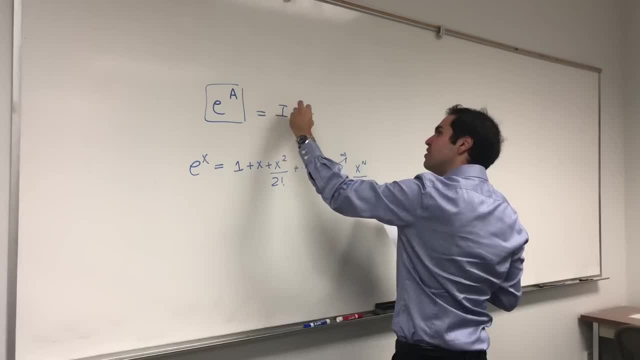 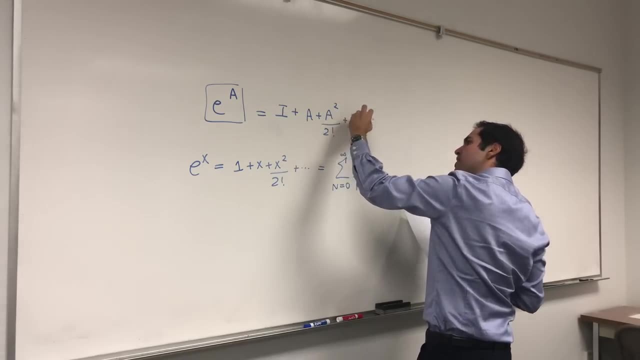 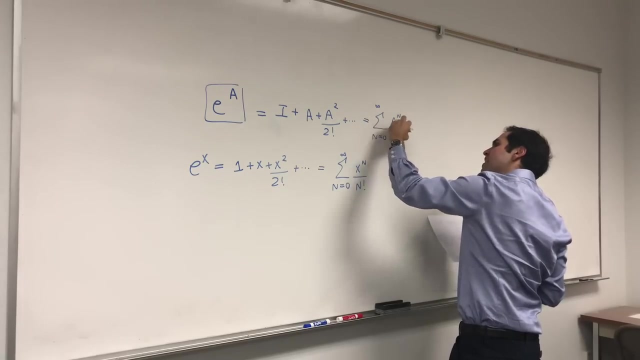 formula 1 is just the identity matrix, x is just your matrix a and then a squared over 2 factorial plus dot dot dot, which in general is the sum from n, from 0 to infinity, of a to the n over n factorial. 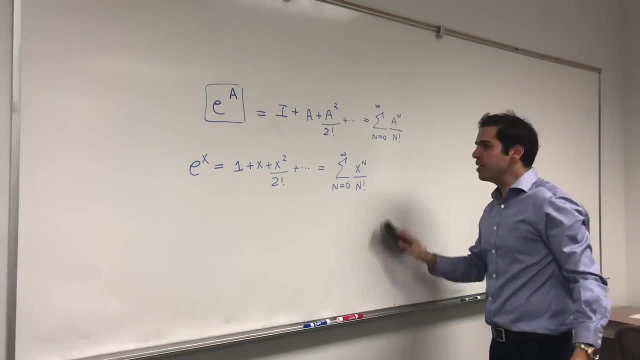 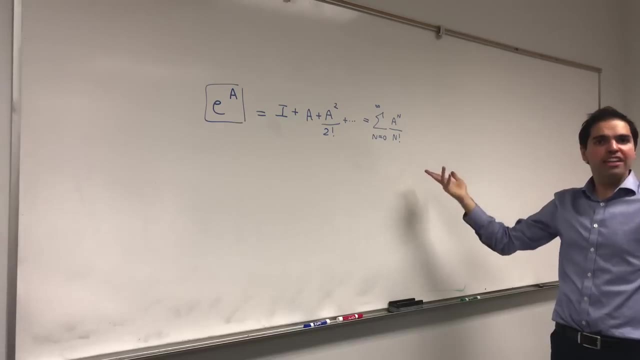 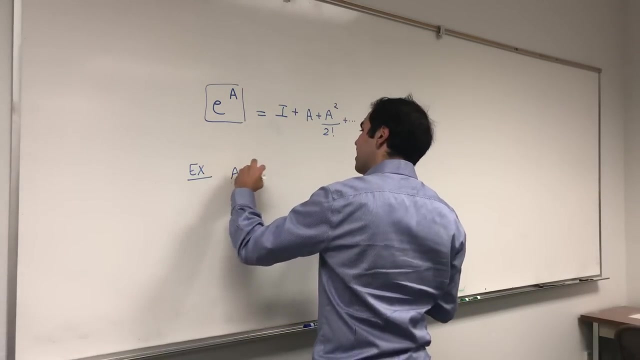 OK, OK. And the question is: well, how do we calculate this? If we're lucky, then the matrix a to the n is easy. So let me give you an example. Suppose a is 0, 1,, 0, 0. Then, well, a is that. 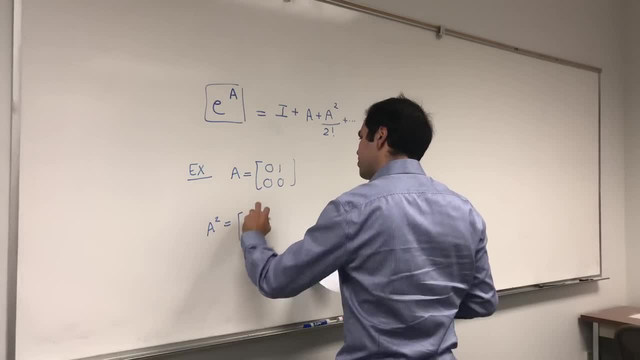 but let's calculate a squared. a squared is 0, 1, 0, 0 times 0, 1, 0, 0 times 0, 1, 0, 0, 0, 0 0.. 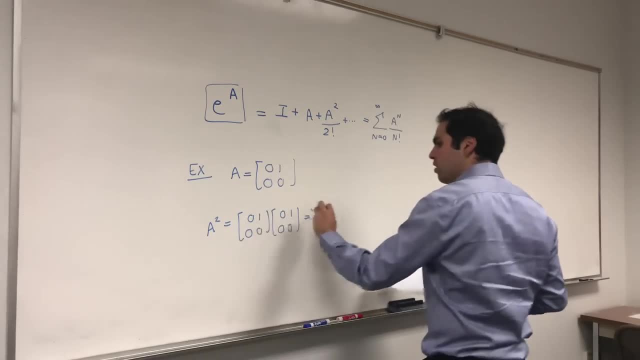 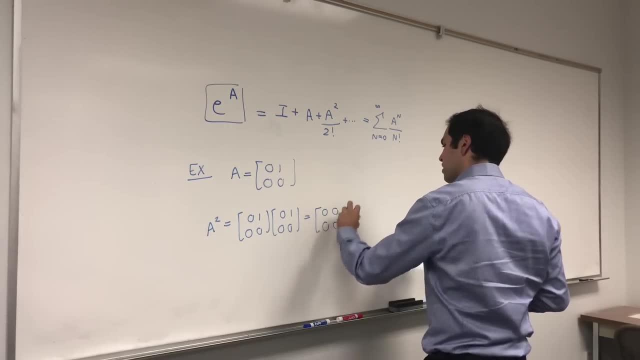 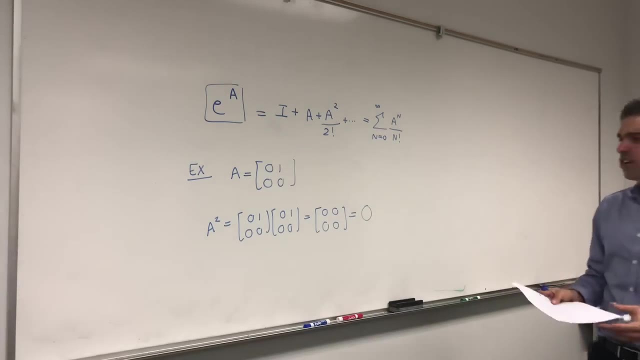 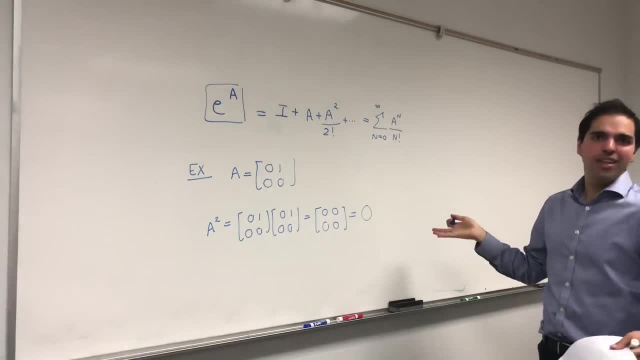 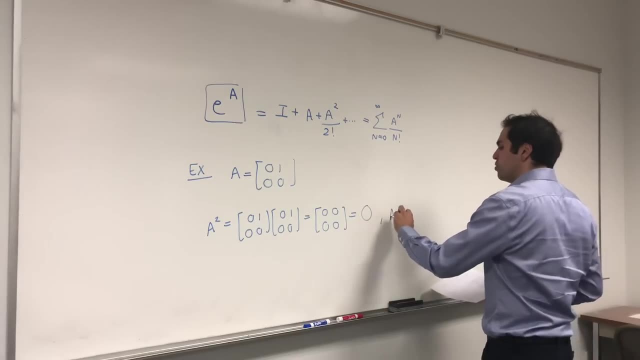 a, which is 0.. a to the 4th is 0 times a cubed, which is 0.. And in particular, any powers of a greater or equal to 2.. 0, 0, 0, 0.. 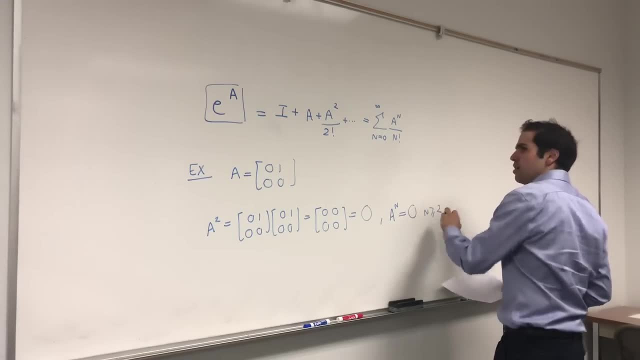 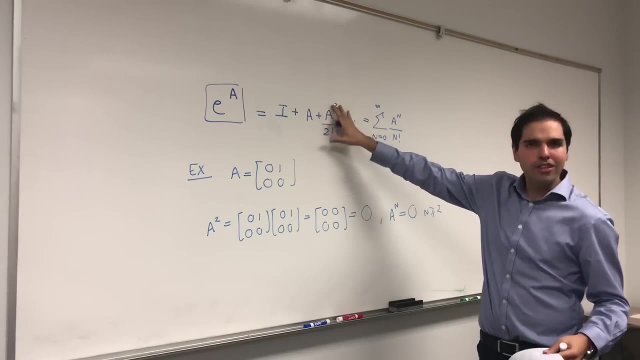 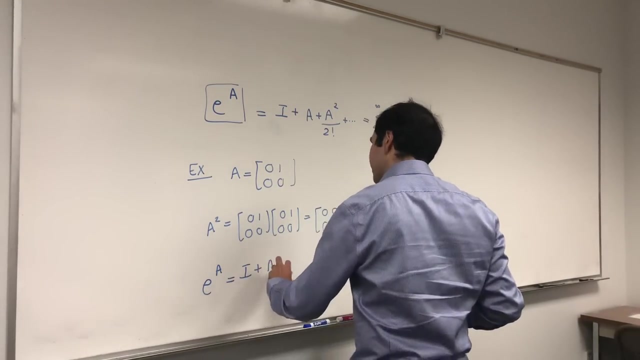 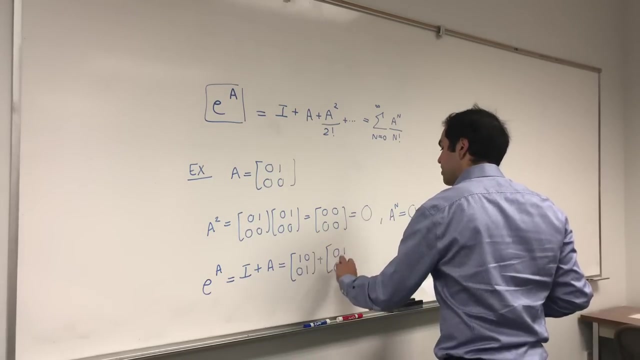 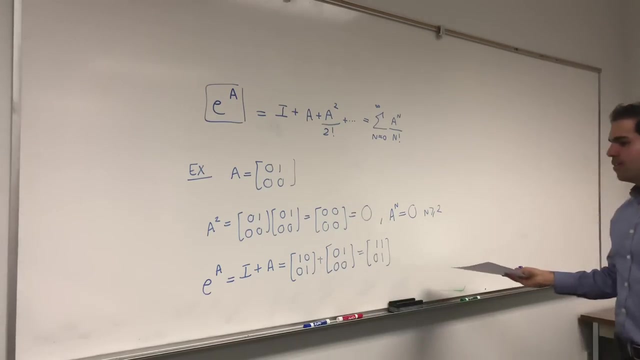 just a zero matrix. so you see, then this infinite series actually just becomes a finite sum. so in this case, e to the a, it's just the identity matrix plus a, which is 1 0 0 1, plus 0, 1 0 0, which is 1 1 0 1, and in general, if some power of a 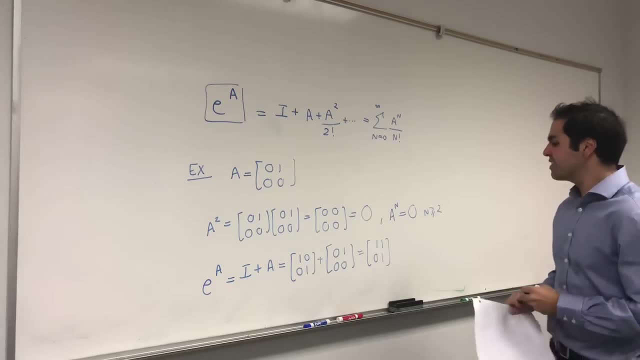 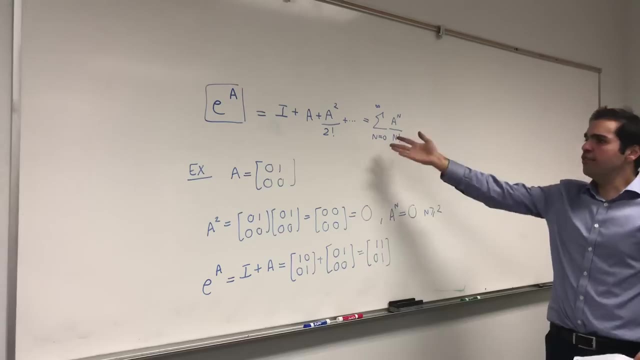 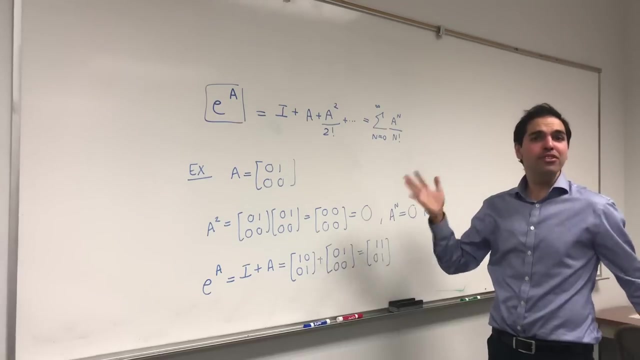 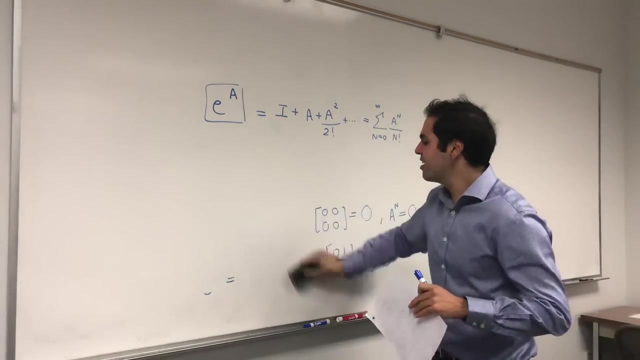 is 0, that's called nil potent matrix. then the x, e, o to the a is easy to calculate because you just use the infinite series just becomes a finite sum. now the question is, though, how do you do it for matrices that are not like that? so what about quote-unquote? the general case, but it's. 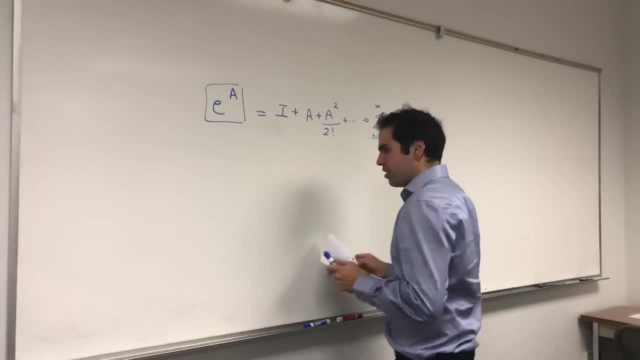 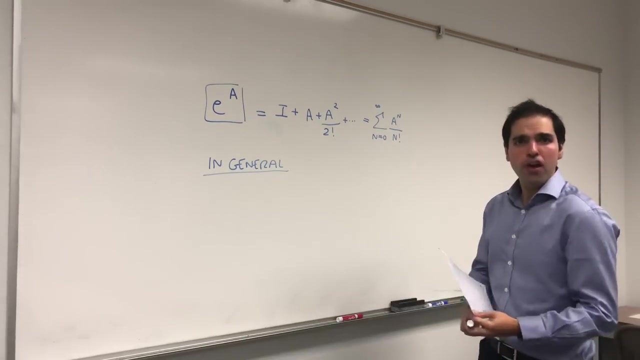 not general, general, but still good. so in general, and I got 100% general because not all matrices are diagonalizable. so in general, and I got 100% general because not all matrices are diagonalizable, but in general, suppose a is diagonalizable, suppose a equals to PDP. 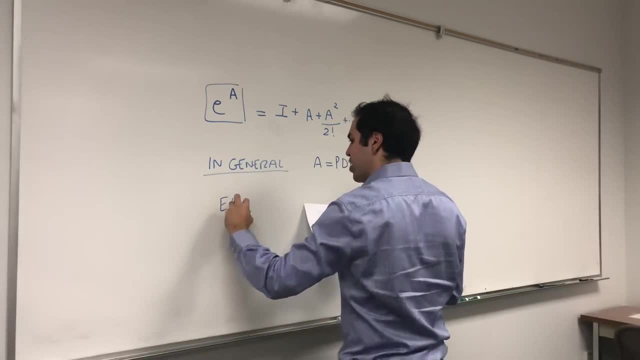 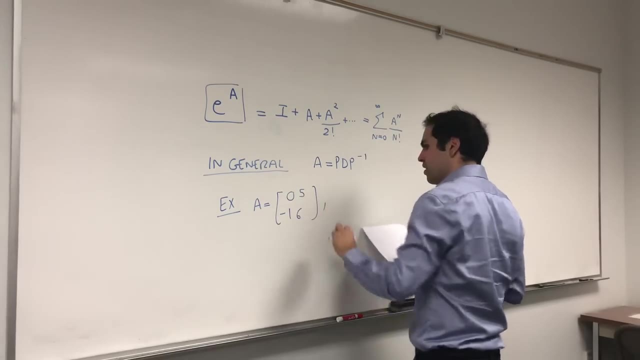 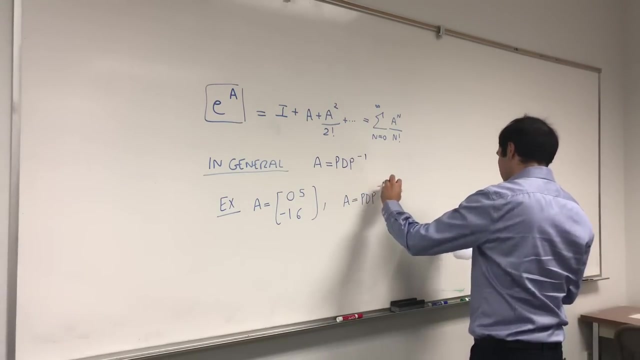 inverse. and let me give you an example. take a to be the matrix 0, 5 minus 1, 6 turns out you can diagonalize this matrix. so a is PDP inverse. where turns out? the eigenvalues are 1, 0, 0, 5. 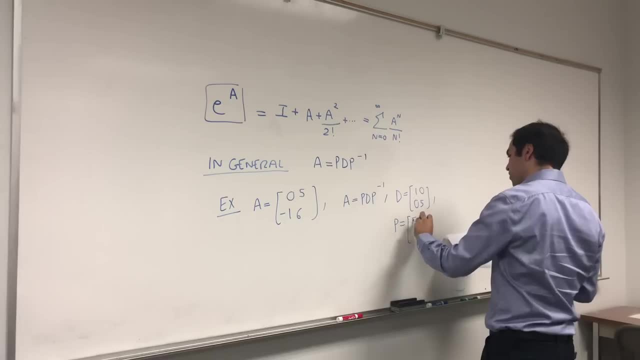 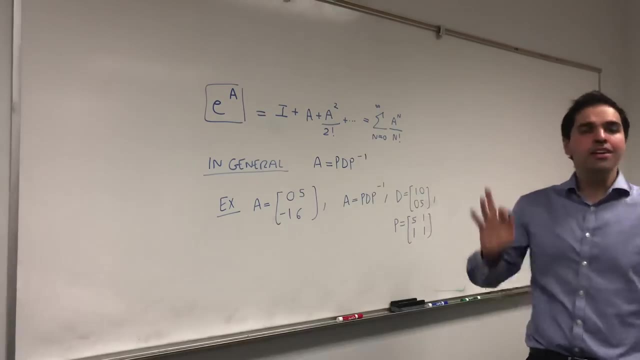 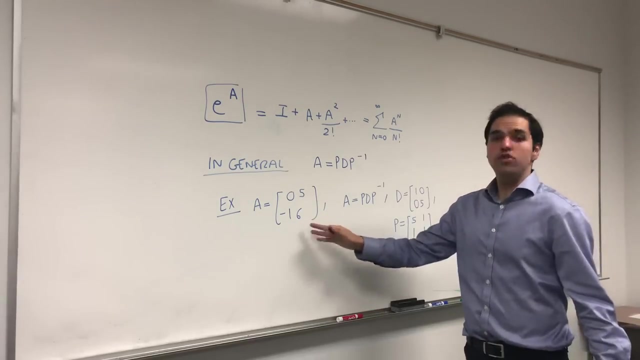 and the eigenvectors are 5: 1 and 1: 1. if you're curious how to find P and D, there's another video I've done. why diagonalize a 2 by 2 matrix and you just use that technique here and you basically find for this matrix the? 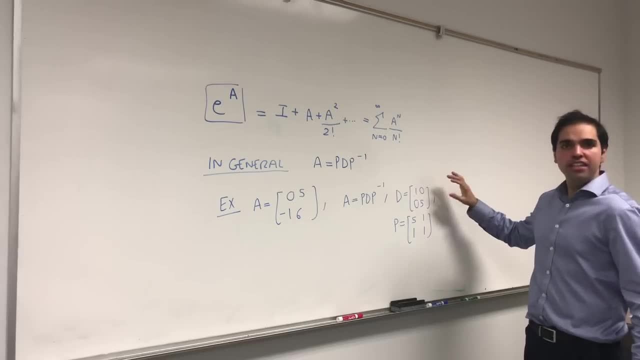 eigenvalues are 1 and 5. so you put in a diagonal matrix with entries 1 and 5 and then you just use that technique here and you basically find: for this matrix the eigenvalues are 1 and 5, so you put in a diagonal matrix with entries 1 and 5 and then 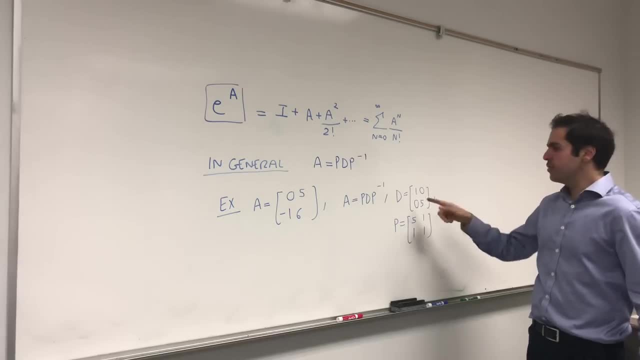 for P you just put corresponding eigenvectors. so, for example, you find: 1 eigenvector corresponding to 1 is 5, 1 and another eigen vector corresponding to 5 is. so this is how you find P and D. but the question is: how can we use this to find? 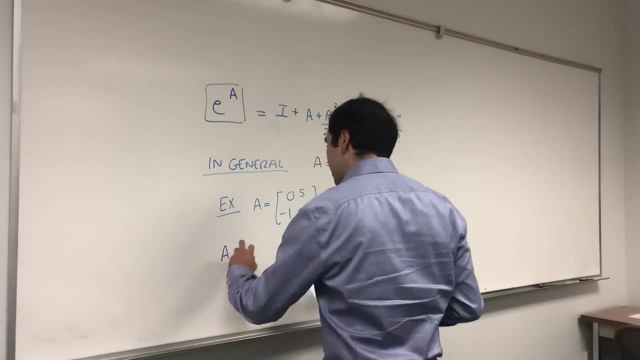 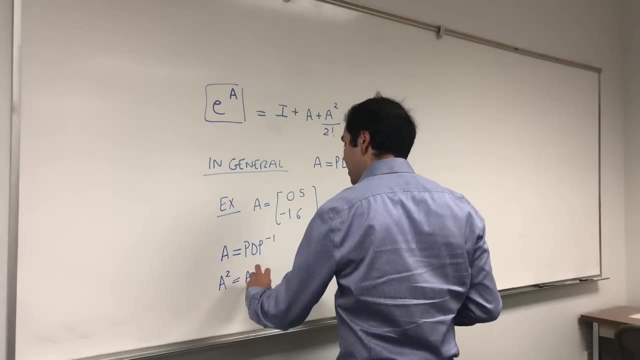 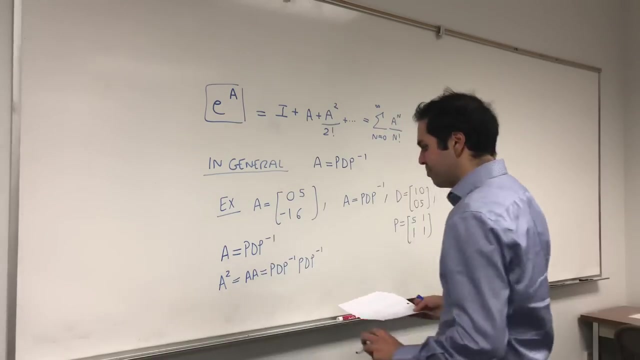 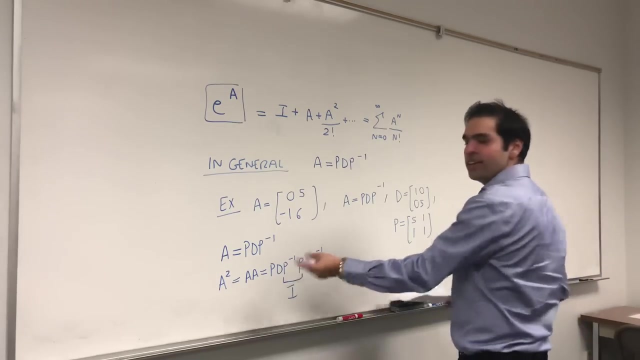 e to the a. now, well, we know that A equals to PDP inverse. well then, a square 3, that's AA and that's PDP inverse, PDP inverse. but notice how nice this is. we get P inverse. P is the identity and the identity in multiplication doesn't do. 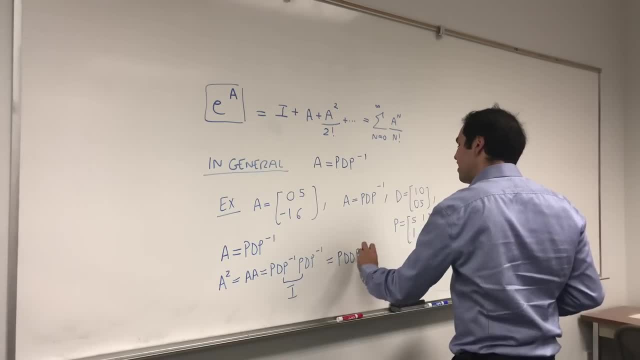 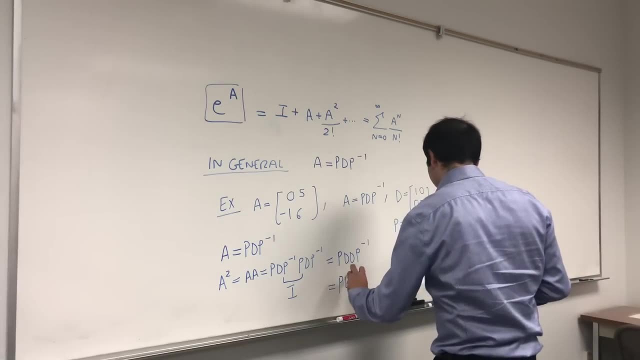 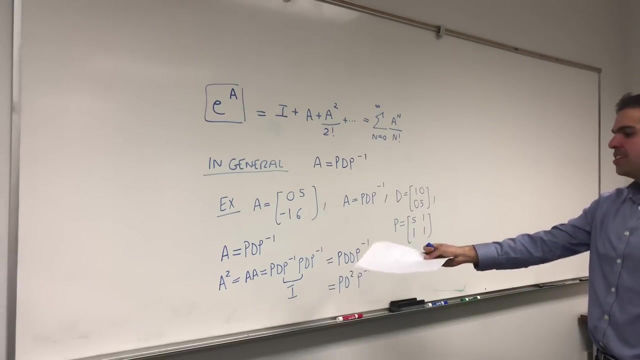 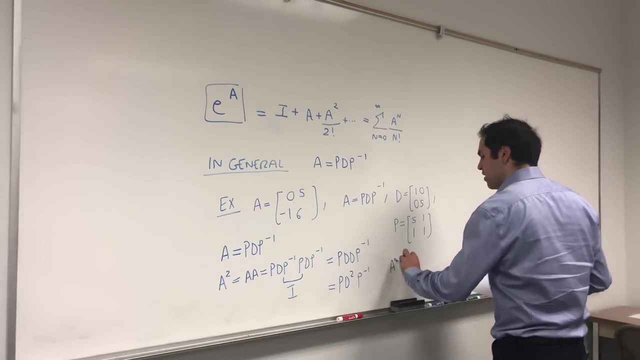 anything. so we literally get PDDP inverse, like PDD, but PDD okay, and we get PD squared P inverse. so you see, a is PDP inverse, a squared is PD squared P inverse. and in general what you get is a to the n is P d to the n, P inverse. and 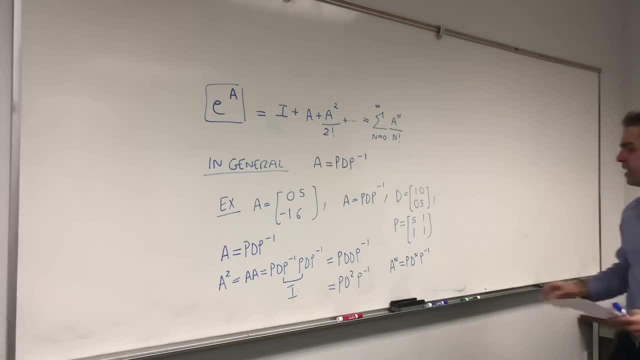 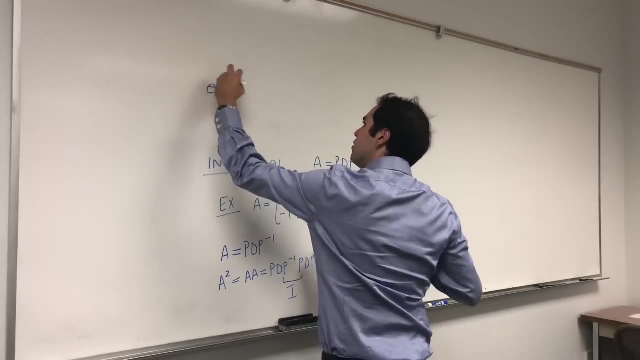 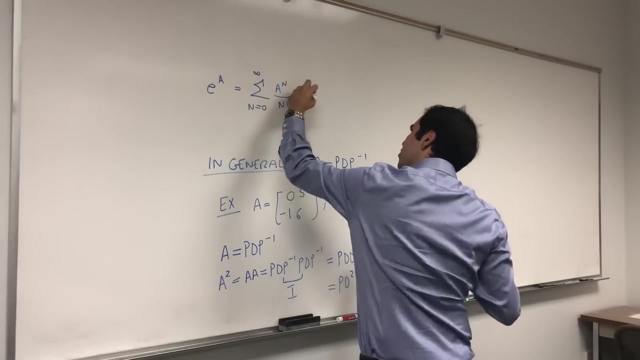 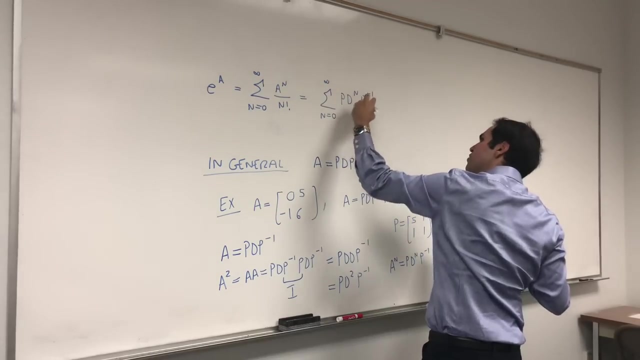 this is super useful in calculating e to the a, because then, what is e to the a, P? remember? by definition, it's the sum from 0 to infinity of a to the n over n, factorial. and that's the sum from 0 to infinity of P, d to the n, P inverse over. 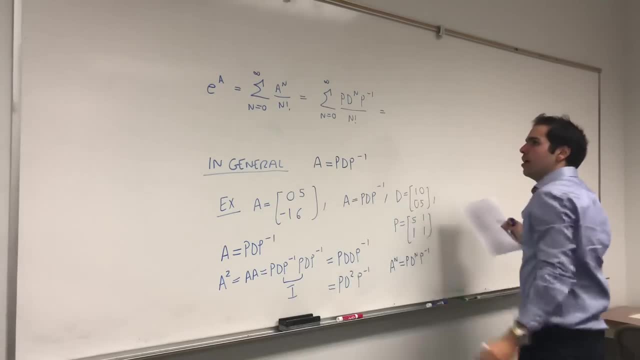 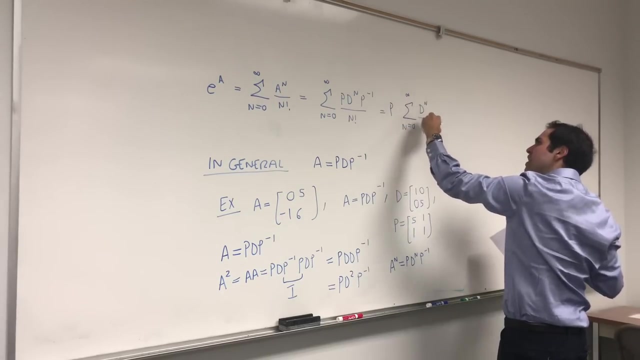 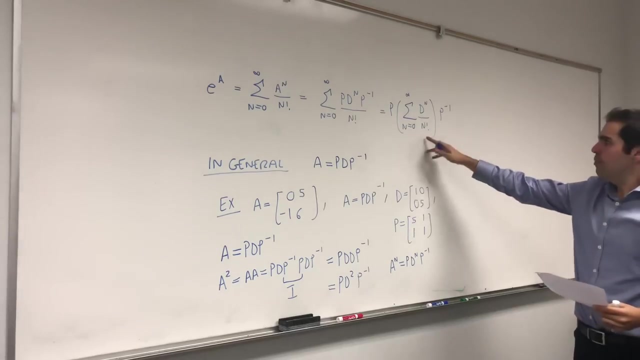 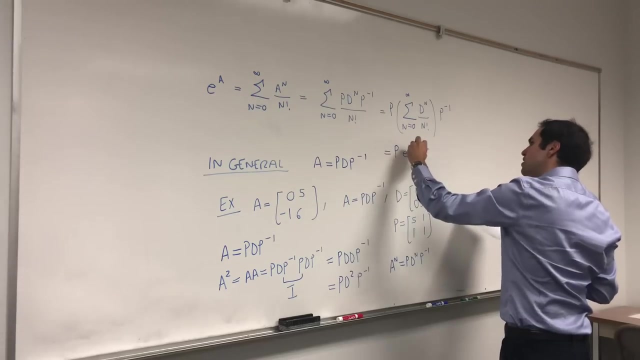 n factorial. and what is that? well, so you see P and P inverse. they act like constants with respect to the sum, so you can actually pull them out. so P some from 0 to infinity, d to the n over n factorial P inverse. but this is just exponential of D, so that's PE to the DP inverse. almost looks like pya, but 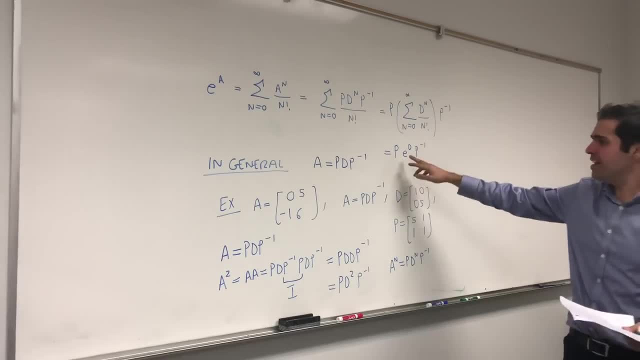 or PDE's I guess. but the point is actuallyいい to the d for D to the e squared. and second thing is if we we Anschluss k, if we use- because we don't know this- actually a e to the D for D squared, I mean pres 해 and pdne plus esqu Não. 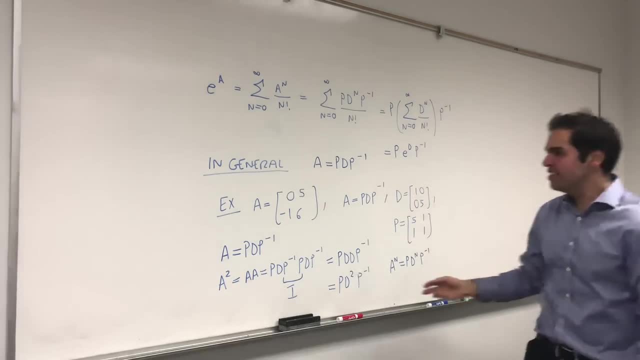 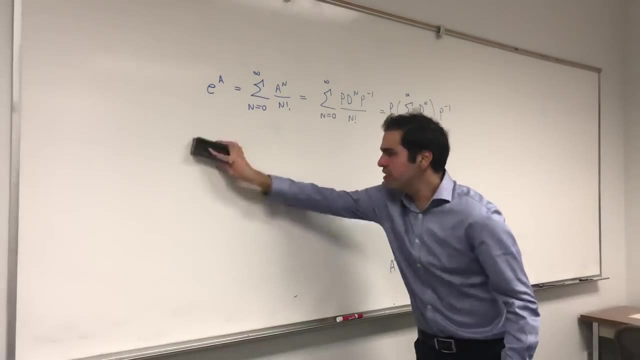 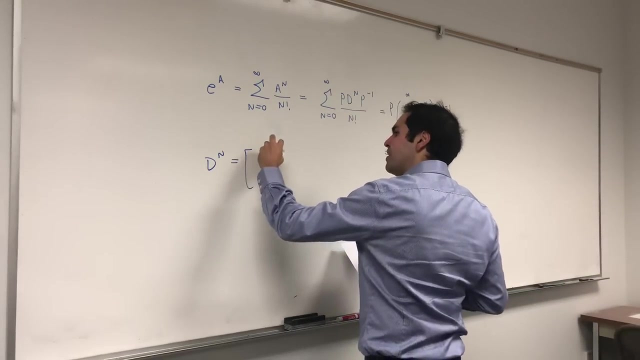 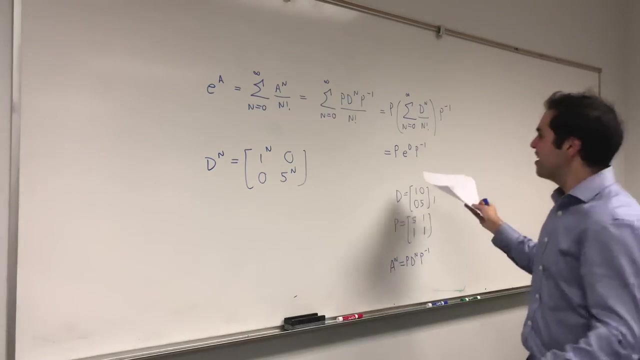 e to the d, for diagonal matrices are very easy to calculate because if you take powers of diagonal matrices, if you take d to the n, it turns out. it turns out. you just raise the entries by n. So d to the n is one to the n, zero, zero, five to the n. 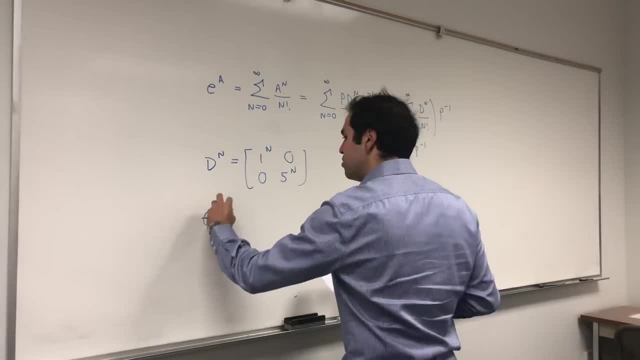 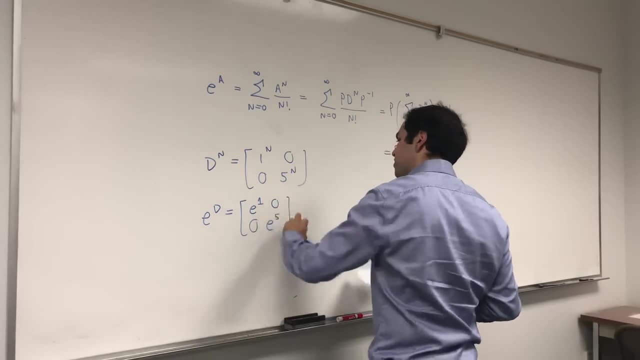 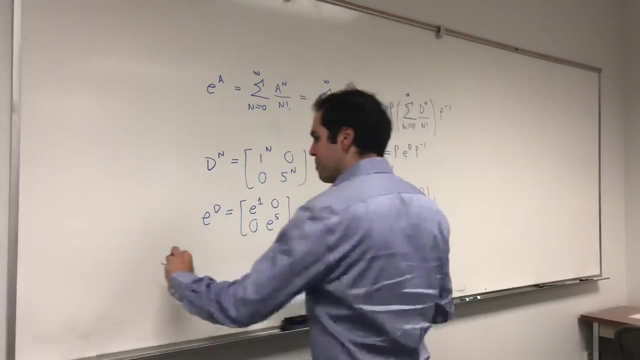 So I'm not gonna prove this, but it turns out, if you do e to the d, that just becomes e to the one, zero, zero e to the five. And let's do this now to calculate e to the a. So remember, a was our matrix. 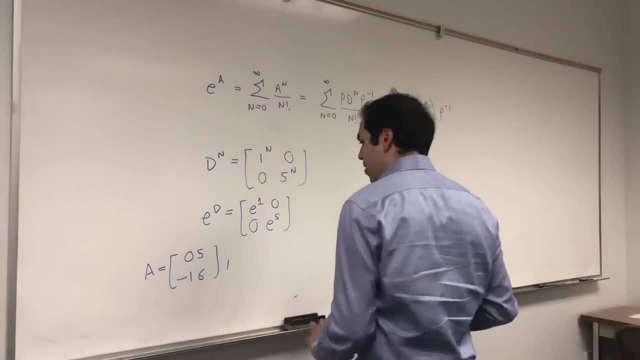 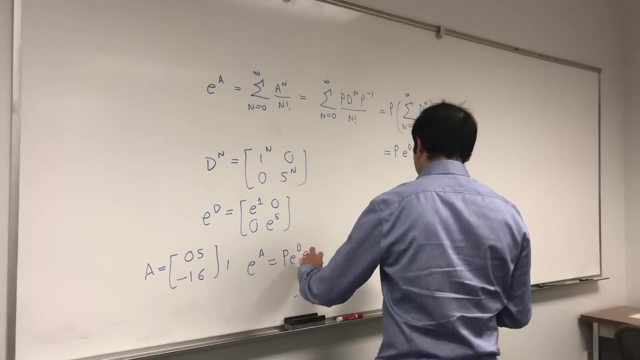 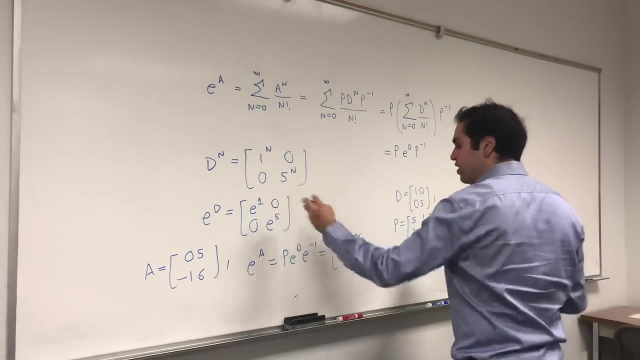 zero, five minus one six. Well then, by what I said, e to the a is then just p, e to the d p inverse, which is just five, one, one, one. now, well, e to the one is e. 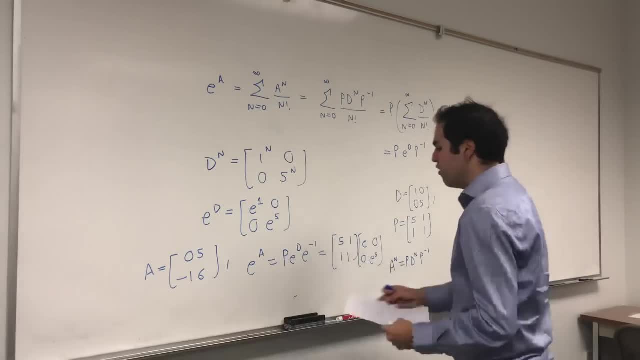 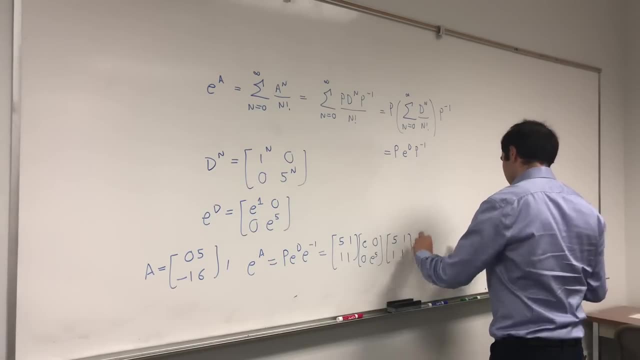 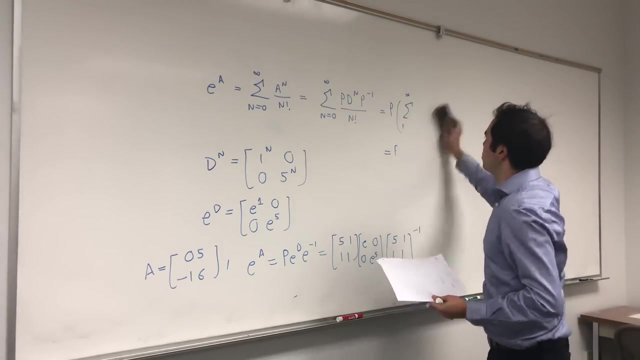 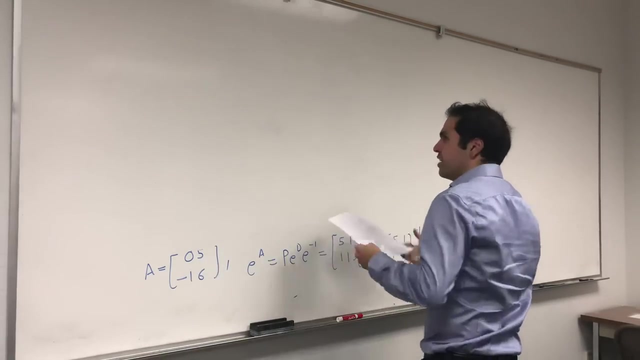 zero, zero, e to the fifth, and five, one, one, one, inverse, Inverse. and then you can just explicitly calculate this, And in fact let's do that. So we get so five, one, one one. 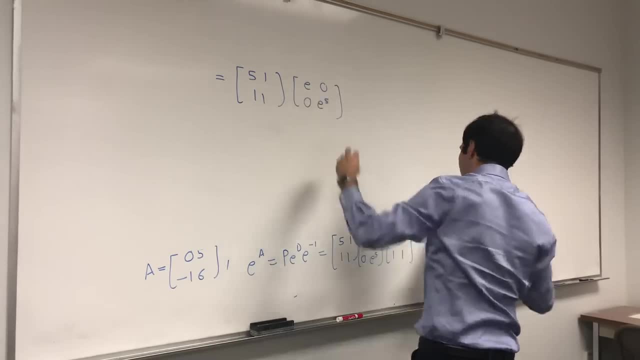 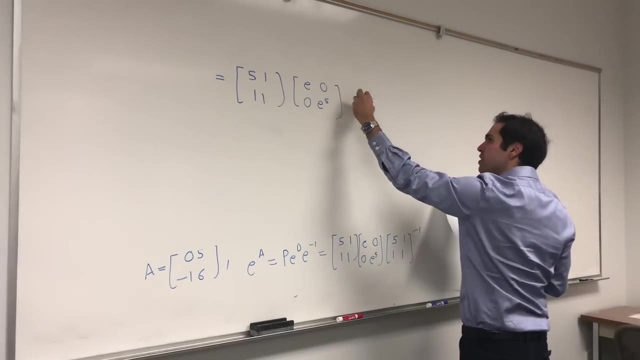 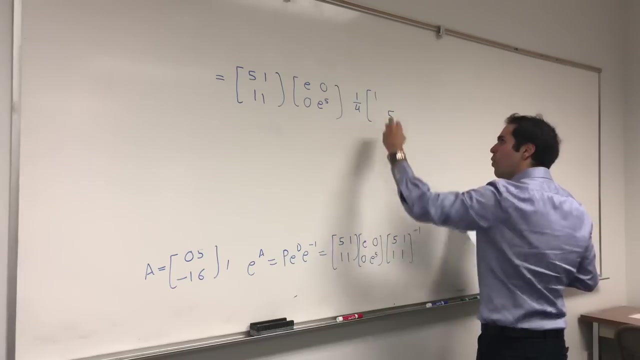 e, zero, zero. e to the fifth, And then two by two- matrix is not too bad to invert, So it's one over the determinant, So one over four, and then five and one, you switch them up. So one and five, one and one, you put minuses. 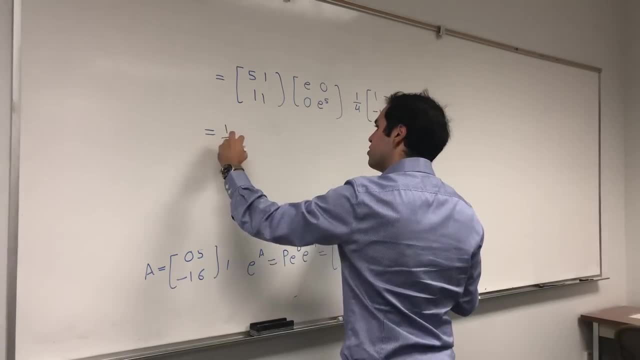 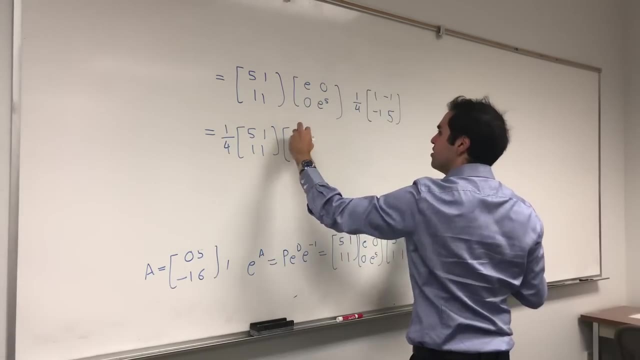 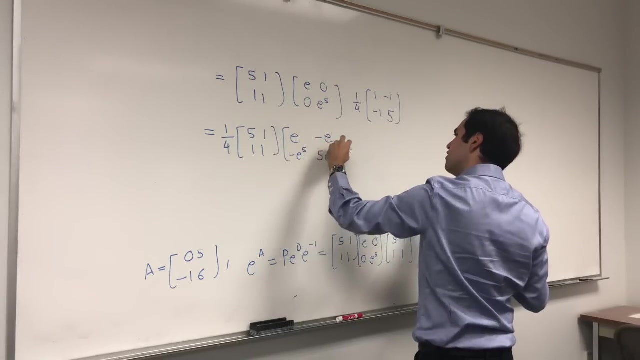 And there you go, And then you calculate this: So one fourth five, one, one one and then e times minus one, So just e, and then minus e, minus e to the fifth and five e to the fifth. 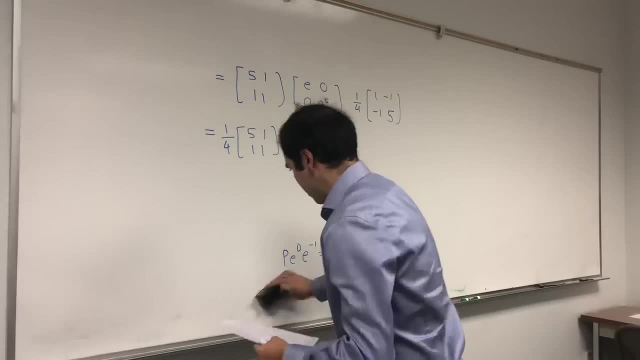 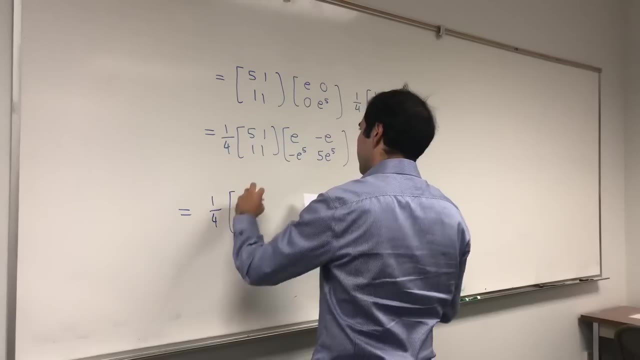 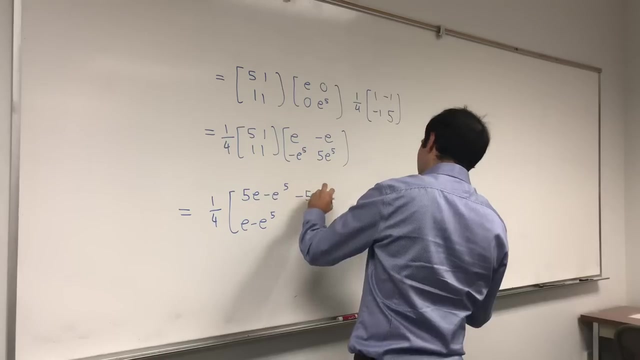 And then you calculate that as well now. So you get one fourth and then five e minus e to the fifth, E minus e to the fifth, minus five e plus five e to the fifth, And minus e plus five e to the fifth. 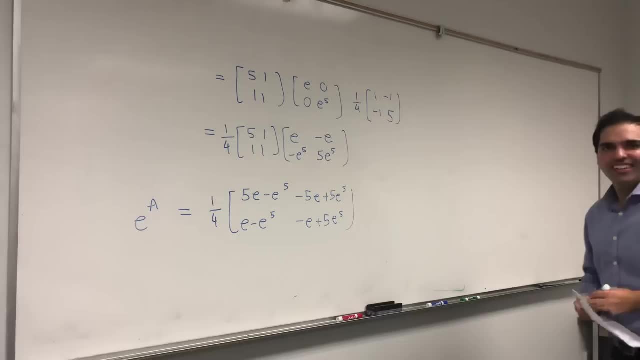 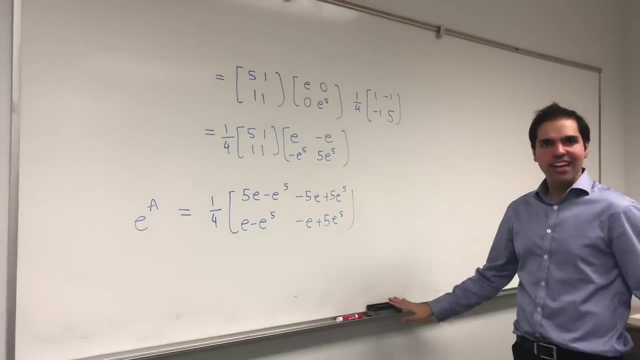 And there you go. This is the exponential of a. How nice is that? And couple of remarks. So how do you do it? if a is not diagonalizable, It turns out you can use the Jordan form for that, And the nice thing is, the Jordan form writes it into a 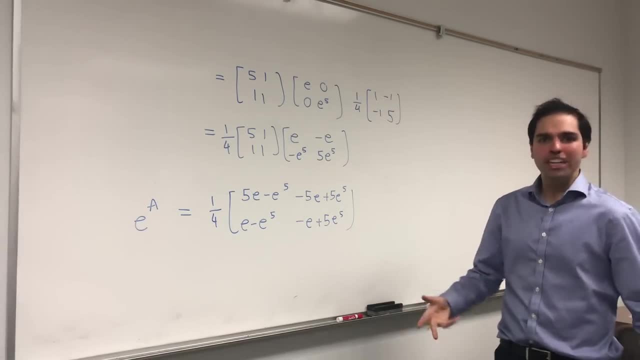 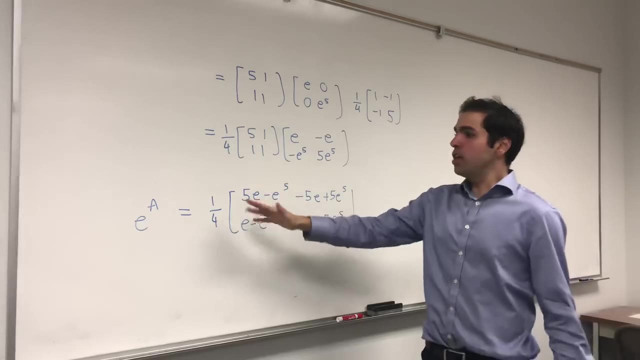 and then you can use the Jordan form for that, And the nice thing is, the Jordan form writes it into a, in terms of those nilpotent matrices where the powers, eventual powers, are zero. Second remark: there's nothing special about e to the a.